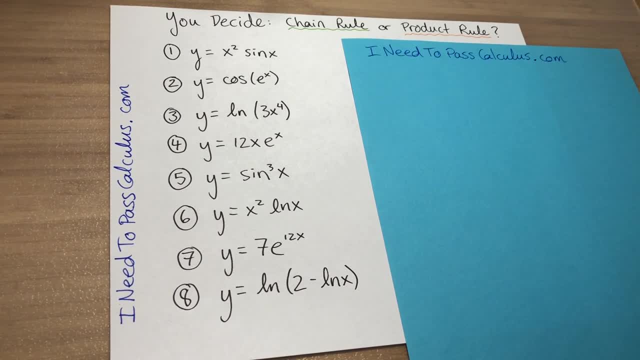 derivatives, and it combines a whole bunch of different rules. it can be really hard to decide which one's the right one to use. So two of the most difficult to choose between rules are the chain rule and the product rule. So today we're going to practice a couple. Feel free to pause right here and try. 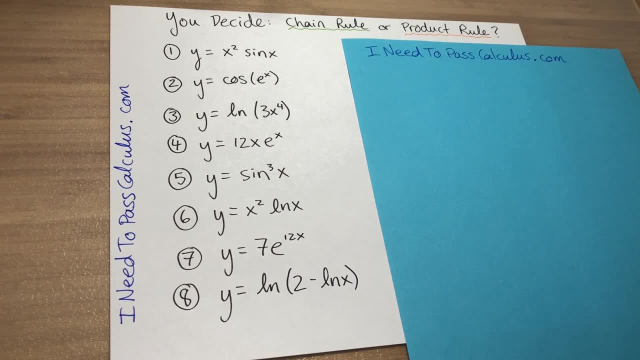 deciding for these eight problems, whether you would use the chain rule or the product rule. Okay, so let's get started For problem one. what you want to do is you want to look at the two problems that you're going to be using, The two main pieces of the function you're given, and you want to see if they can. 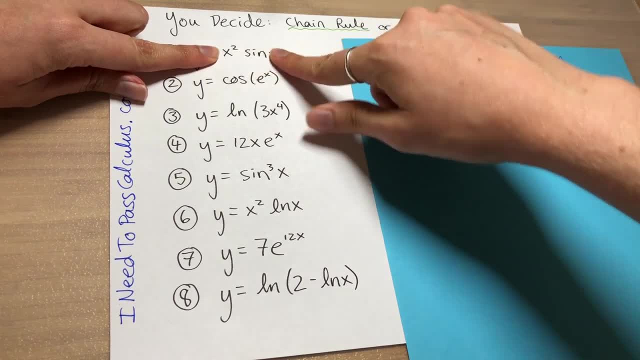 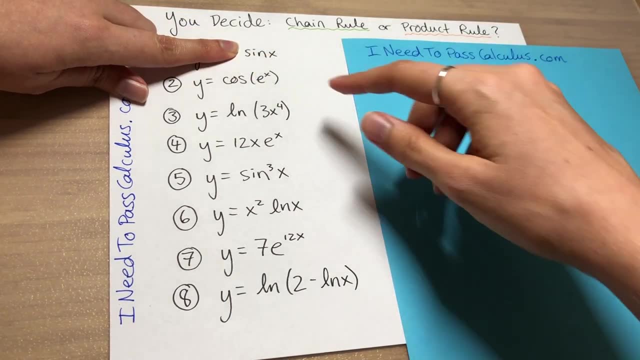 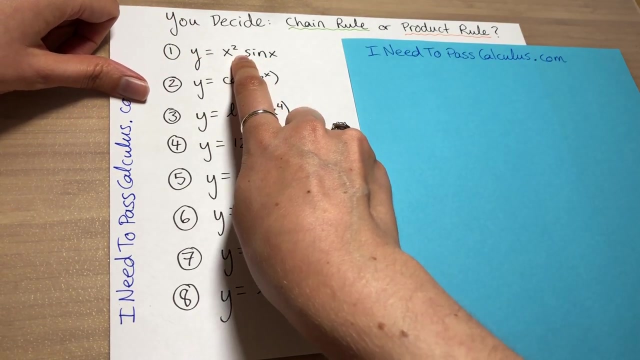 survive on their own. So the two main pieces are x squared and sine x, and when you cover up the other part, there are standalone functions that could be their own problem. So that means that these are glued together with a product, and so you would use the product rule for this problem. 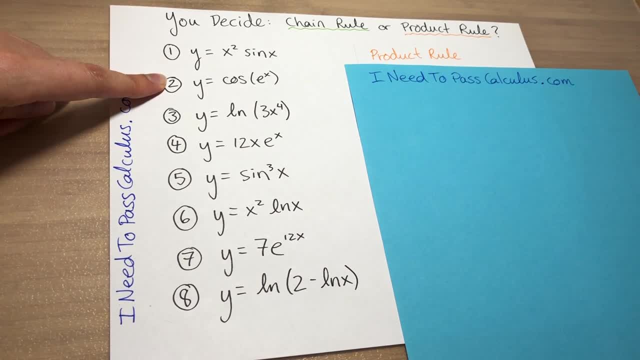 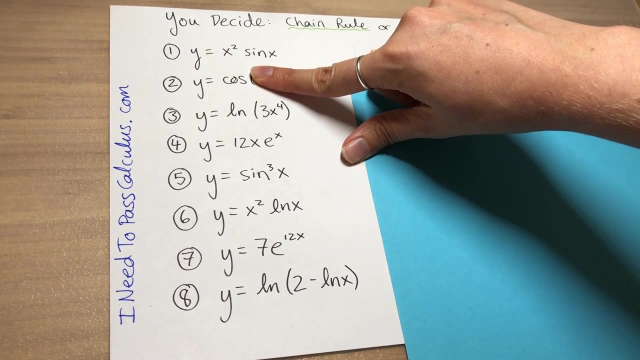 Okay, so for problem two now. our two main pieces of this function are the cosine and the e to the x. And if we cover up the e to the x and just look at the cosine, that's just a COS, It's just cosine, but without any variable there. So 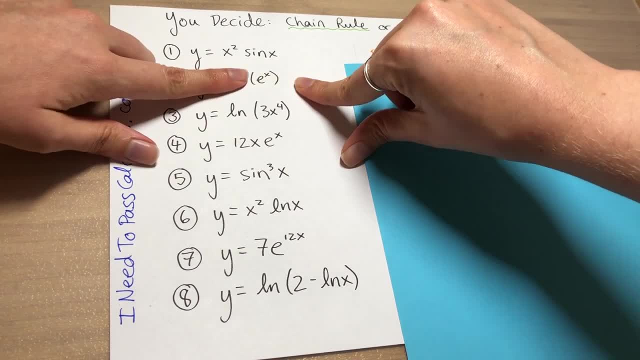 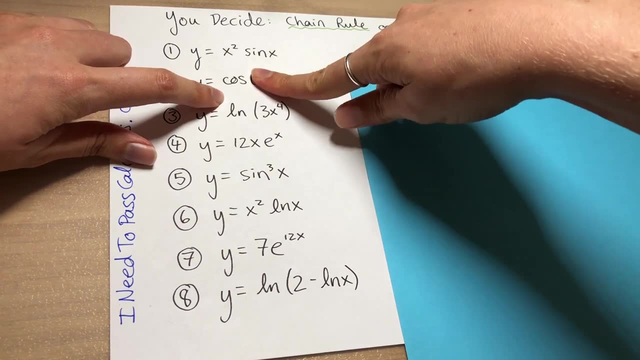 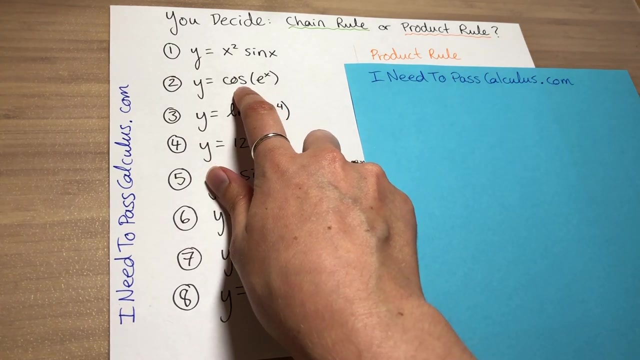 that's actually not a standalone function. If we cover up the cosine part, we get e to the x, which is a perfectly fine standalone function, But because both parts can't stand alone as their own function, that's a hint that this is actually chain rule. This is composition of functions, and so you have. 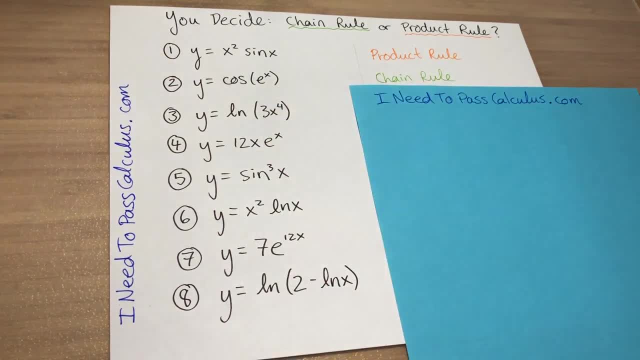 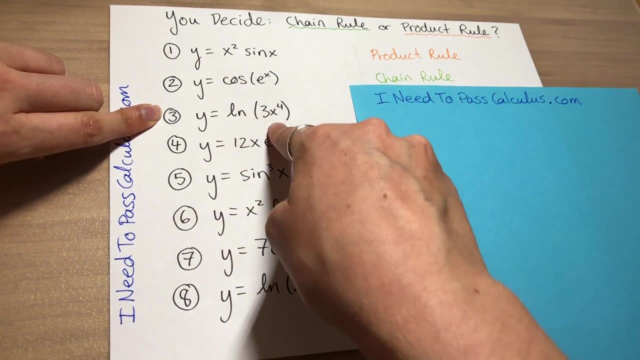 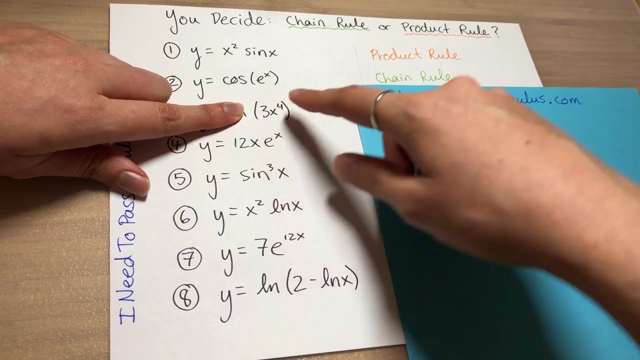 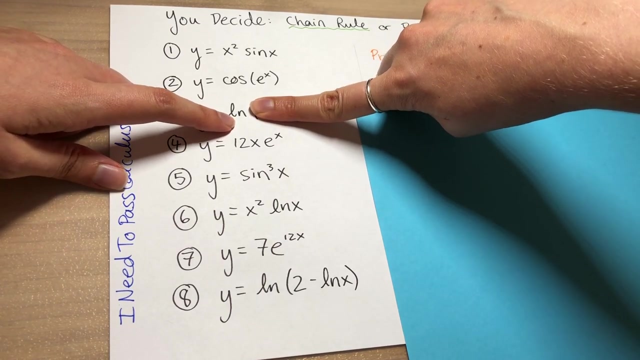 to use the chain rule. Okay, so problem three: Let's look at each of the main parts of this function and see how it is put together. So one of the parts is three- x to the fourth, and the other part is ln, But the ln when it's written like this, without any variable. 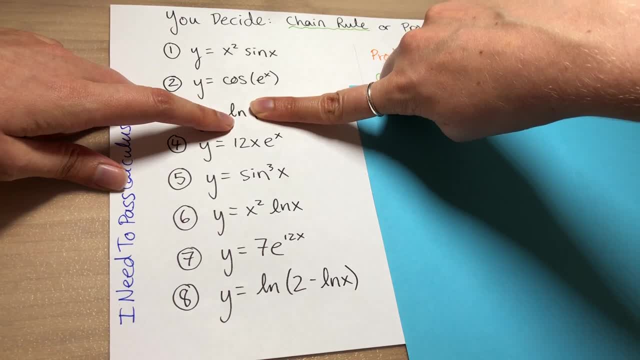 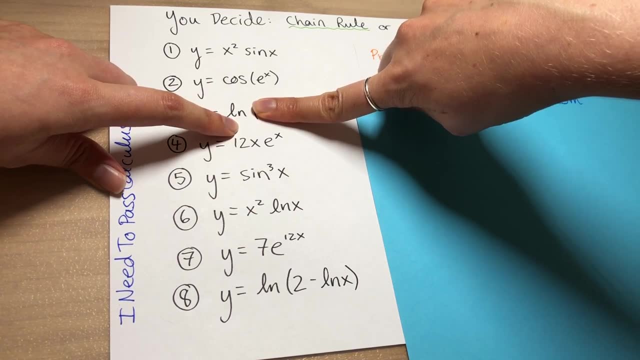 is not standalone. That's not a function that can stand by itself. The three x to the fourth is fine, but the fact that the ln is just an ln is a hint that this is actually a chain rule problem. These functions are nested together. 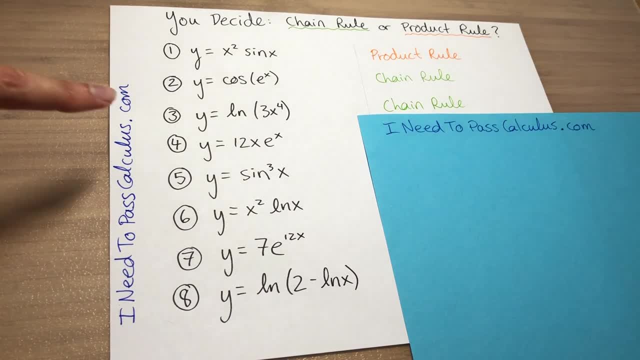 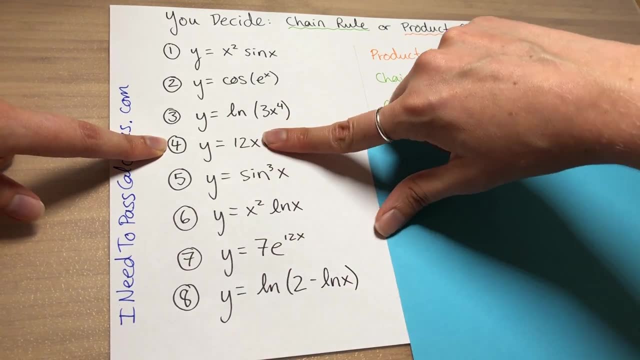 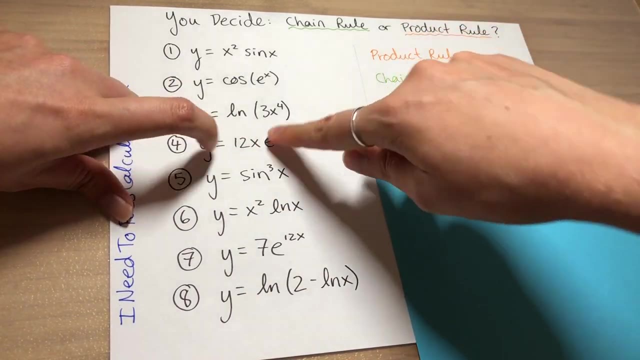 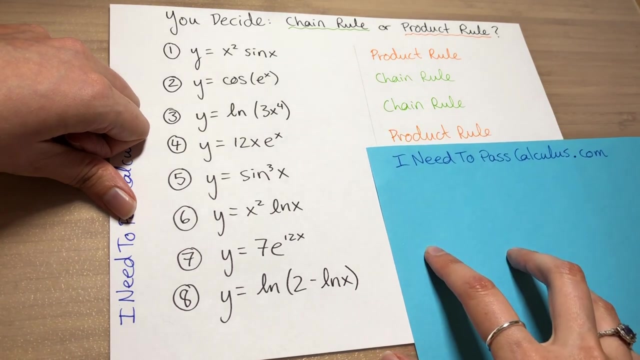 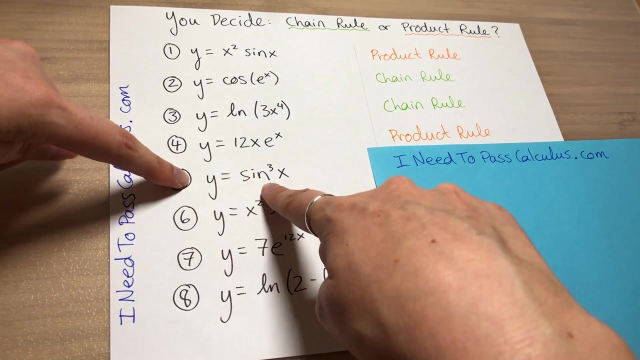 Okay, now problem four. If we look at the, the two main parts of this problem, We have 12x and we have e to the x, And each of those actually is its own standalone function. So these guys are glued together with multiplication right there. So this is a product rule, derivative Problem 5.. Now the most common way to rewrite: 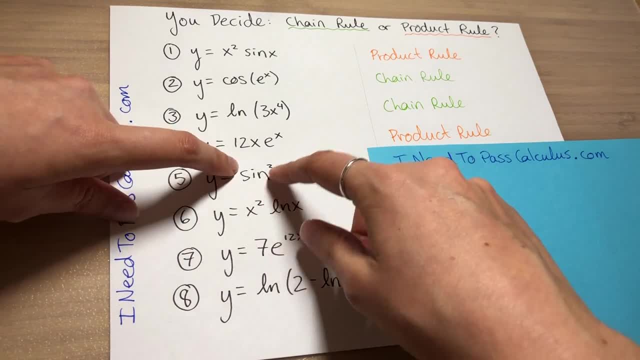 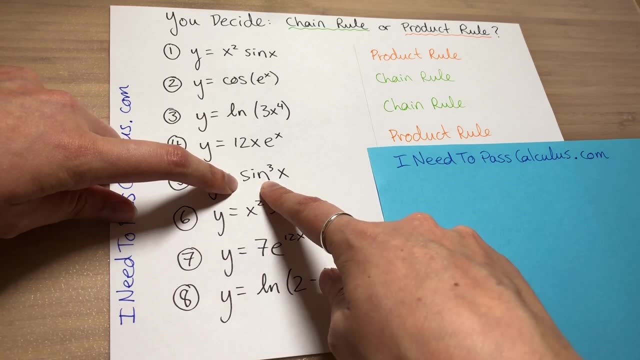 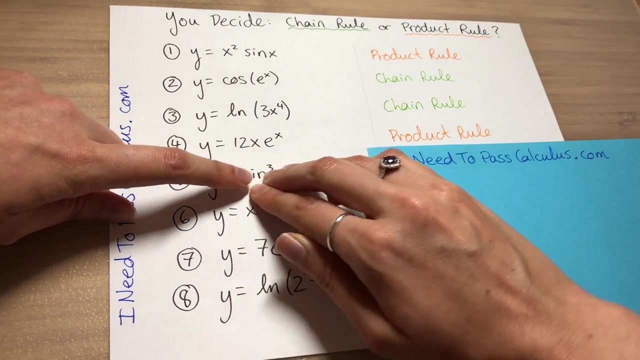 this problem would be with parentheses, where you have parentheses sine x to the third outside of the parentheses. This is just another notation for that. And so your two main parts of this function are the sine x part and the to the third power part. But if you look at the to 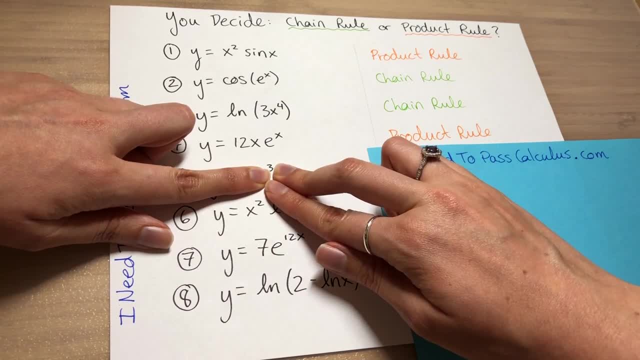 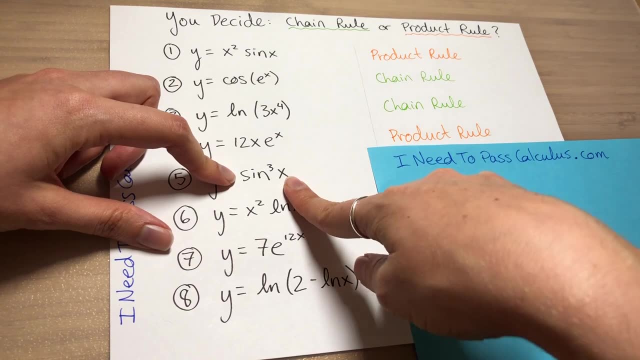 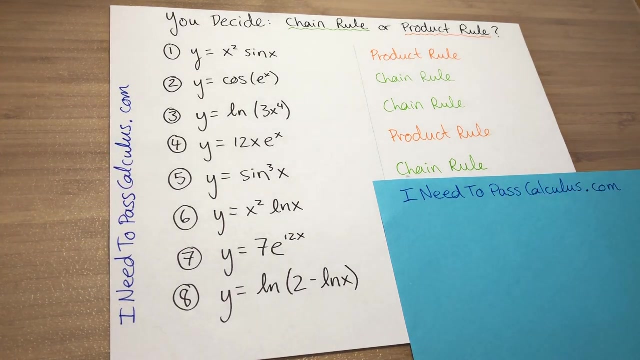 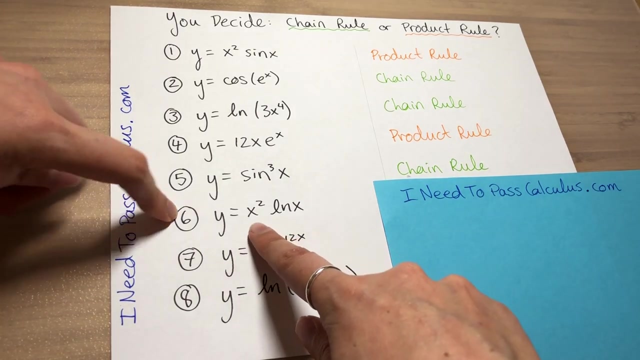 the third power, part a little. 3, floating in midair, is not a standalone function by itself. The sine x is fine. This is a hint that this is actually nesting of functions and it is the chain rule. Okay, problem 6.. So for this one we look at our two main parts of our function. We have an x squared. 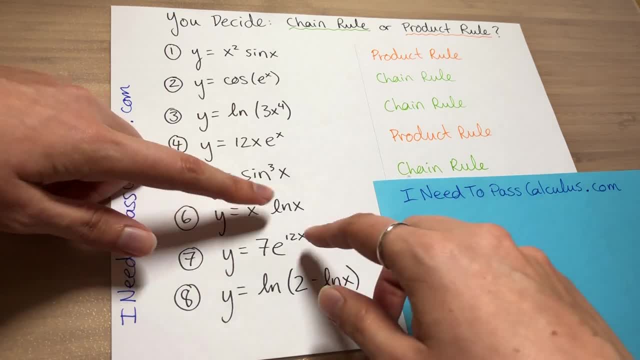 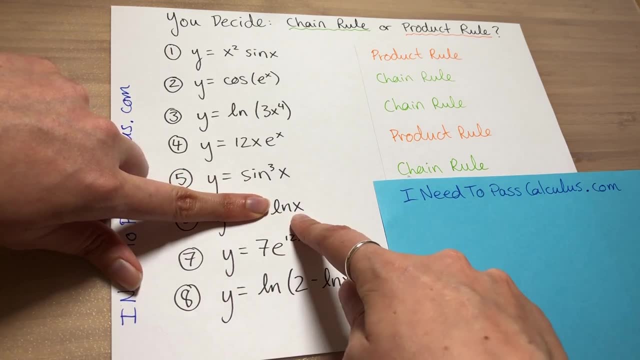 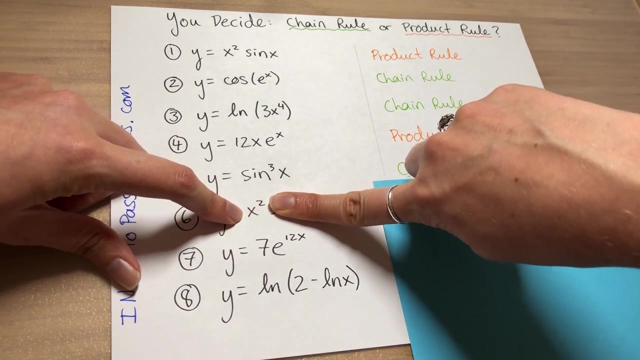 part and we have an ln x part And in this case, unlike the previous ln problem, this guy is actually a full ln x. So this guy by itself is a standalone function and the x squared is a perfectly fine standalone function. So that's a hint that these guys are glued together with multiplication and 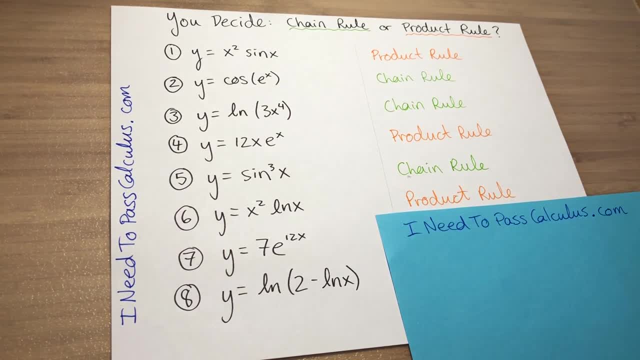 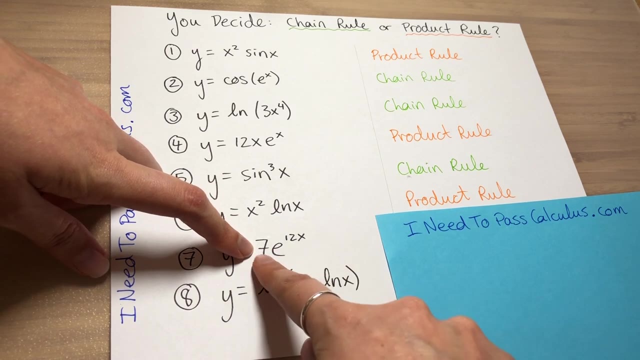 this is going to be a product rule, problem Okay, and problem 7. If you look at this problem, make sure if you ever have a number out front of your function, don't let that trick you into doing product rule Anytime. you have a plain old number.